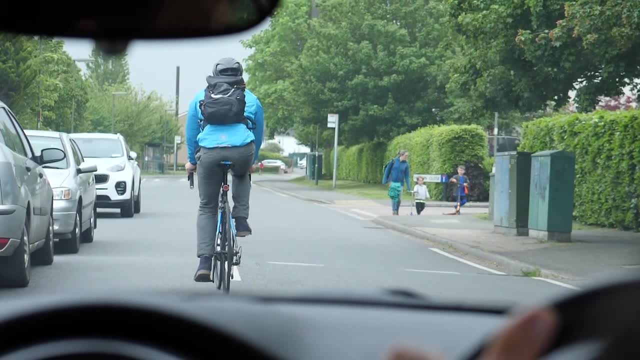 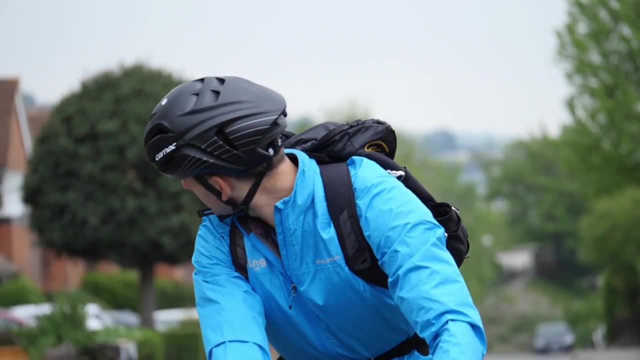 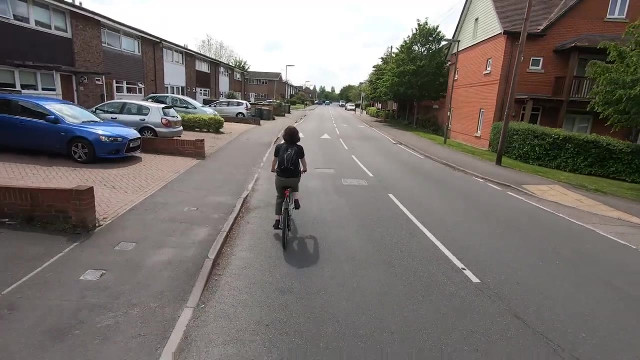 arm's length away from the kerb. When cycling past parked vehicles, be at least a car door's width away from them. Always check over your right shoulder before moving to ensure it's safe to do so. Passing side roads: When passing side roads on your left, check over your right shoulder. 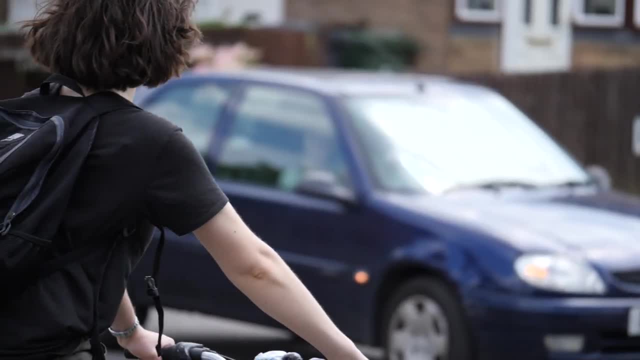 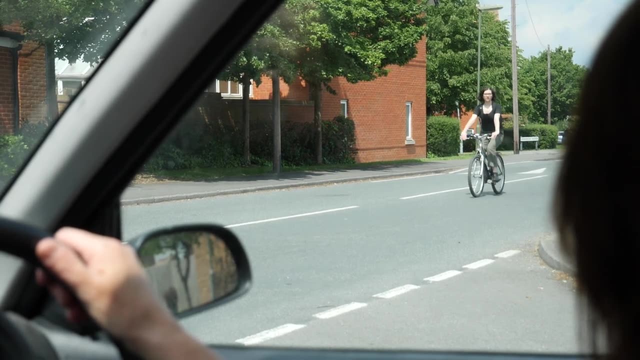 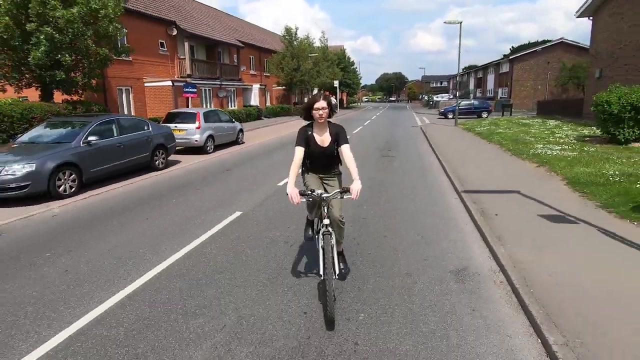 before moving into a more central position. Check the junction for emerging traffic before passing it in the central position. Once you have safely passed the junction, check over your shoulder before once again passing over the junction, again cycling at least an arm's length away from the kerb, Turning right from a 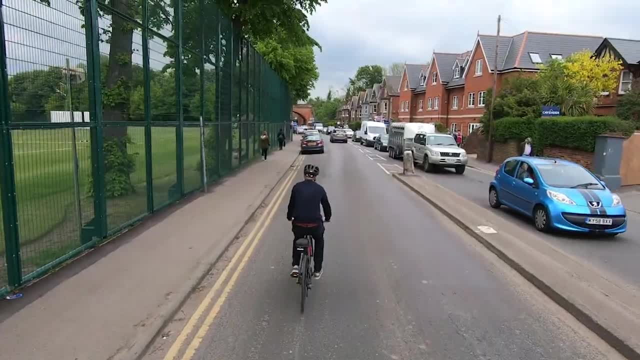 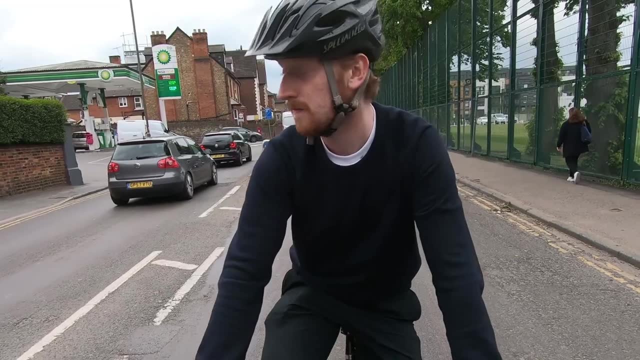 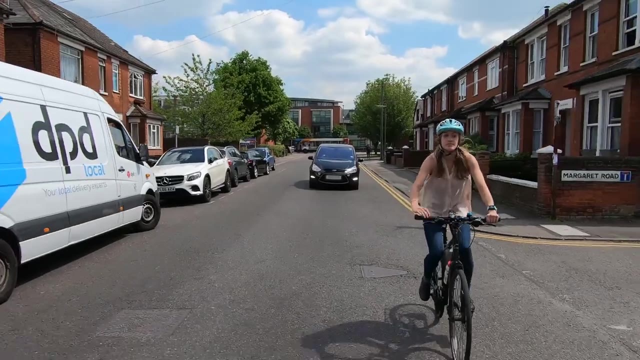 major to a minor road, While still a good distance from the junction. position yourself at least an arm's length away from the kerb. Look over your right shoulder to check if there's anyone behind you. If there is traffic behind you, try and make eye contact with the driver before clearly signalling and. 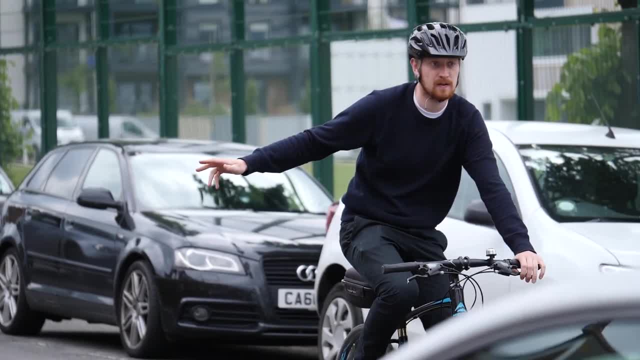 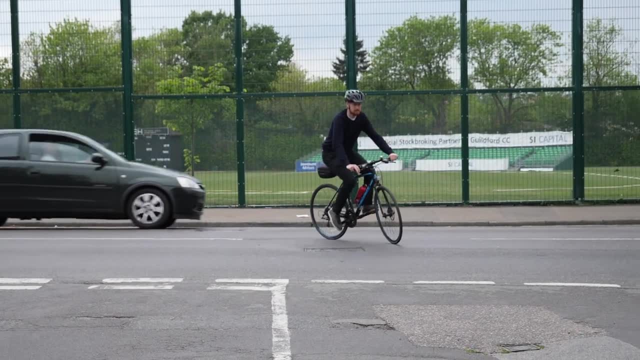 moving out into the right-hand side of the lane. As you near the junction, look for oncoming traffic and be prepared to give way. If it's safe to do so, perform the turn. However, if there's oncoming traffic, stop near the centre of the. 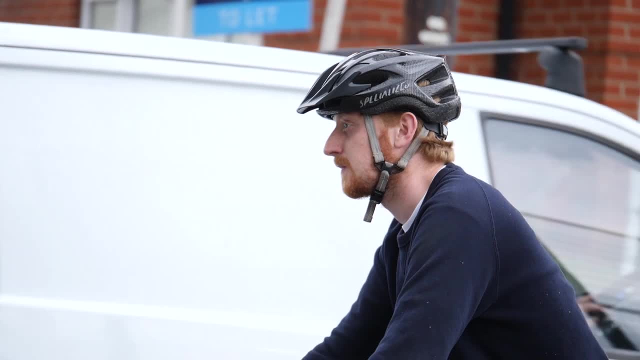 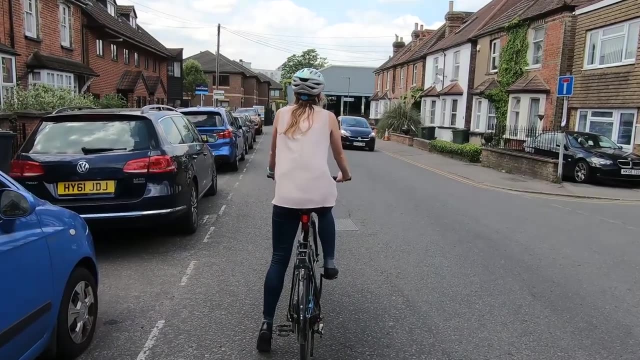 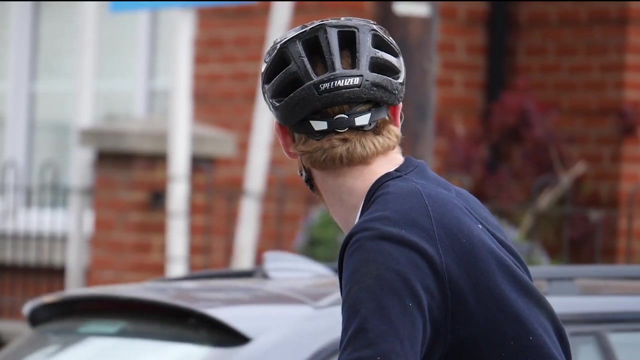 junction you're entering. Keep checking ahead for oncoming vehicles. Allow traffic to flow past your left if there is space to do so, but don't be afraid to take the central position, even if it means that vehicles cannot pass you. Once the way is clear, look over your right. 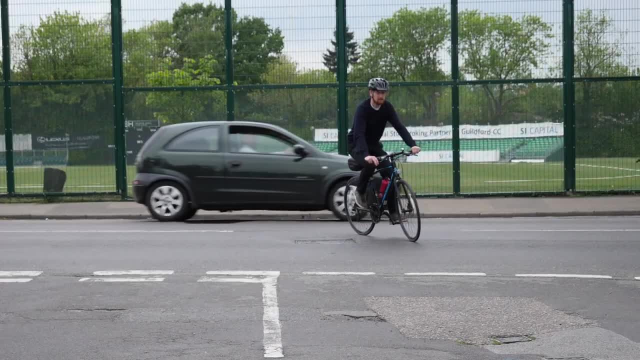 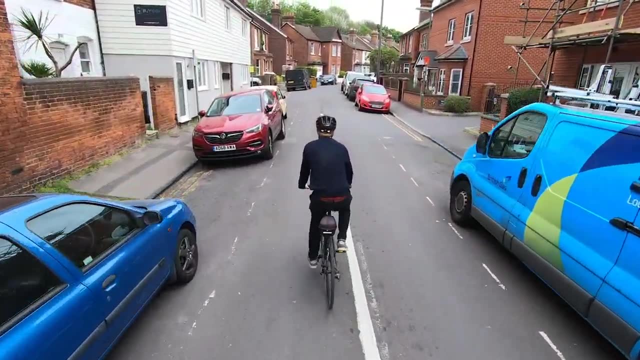 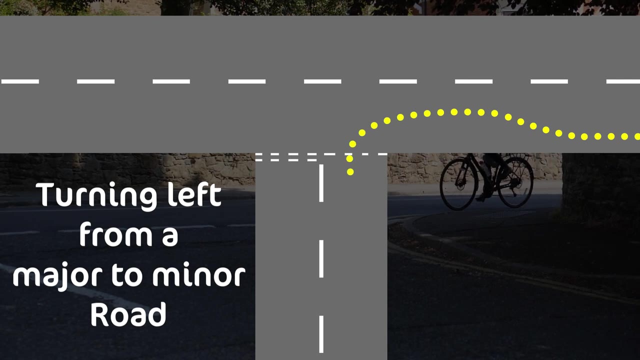 shoulder and perform the turn aiming for the center of the lane you're entering, Once you're safely away from the junction cycle, at least an arm's length away from the kerb Turning left from a major to a minor road. As you approach the junction, check 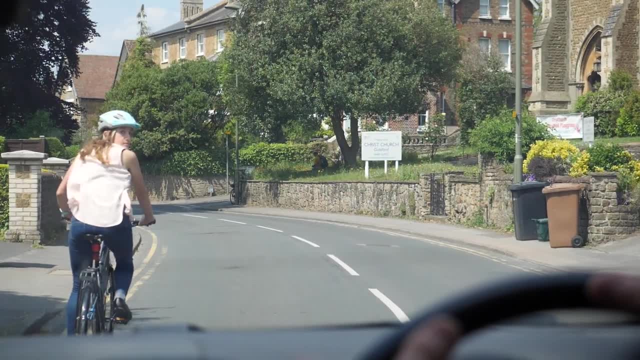 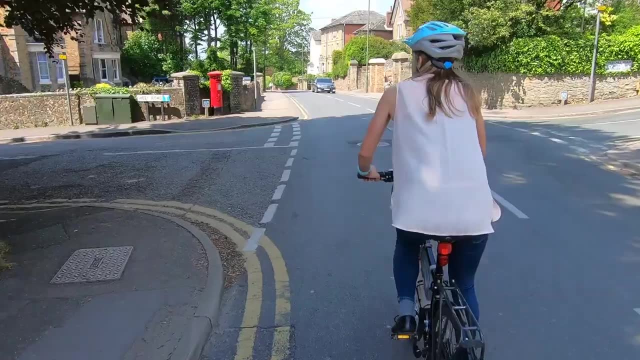 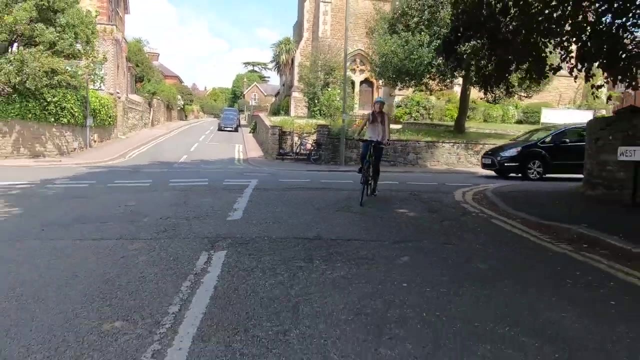 over your right shoulder and try and make eye contact with the passenger, with the driver behind you. then move out into the centre of the lane and indicate left. Look over your left shoulder to check for undertaking cyclists, then perform the turn aiming for the centre of the lane you are entering.